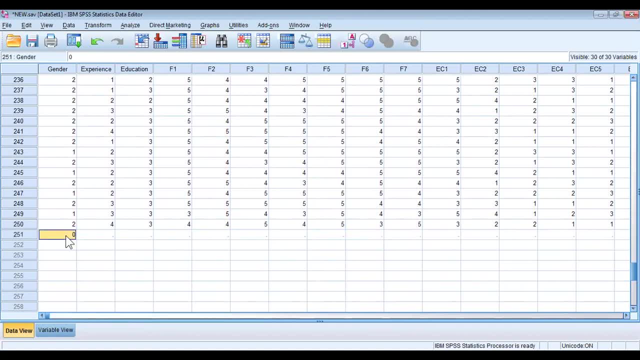 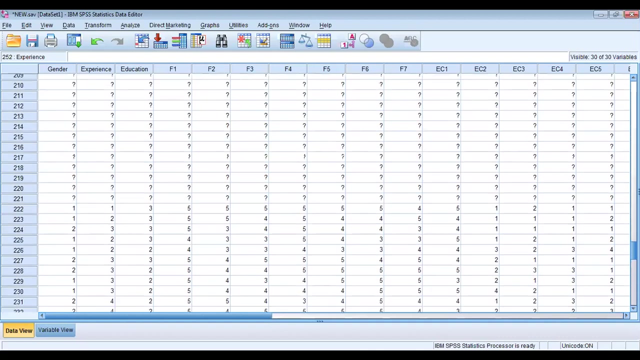 if you have typed something here and then you have removed it. now this 250 first bar is still highlighted, Okay, Okay, So you can see here it has some data, although you've already deleted it, but it is showing as it has some data. So we'll keep it like this and we'll see what to do now. 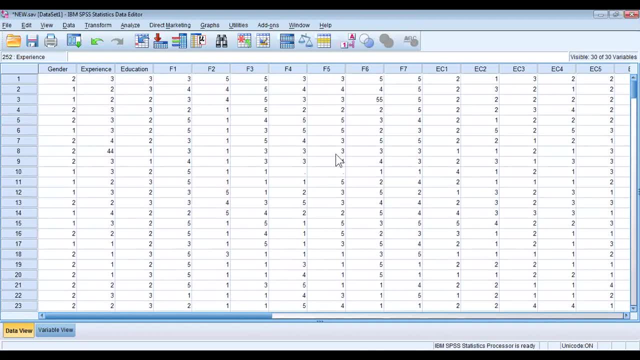 In this video we'll be mainly talking about the sifting of data, or cleaning of data. or you can say we'll be finding the typos in our data, or you can say that we'll be finding the outliers in our data. So, while typing the data manually, most of the people, most 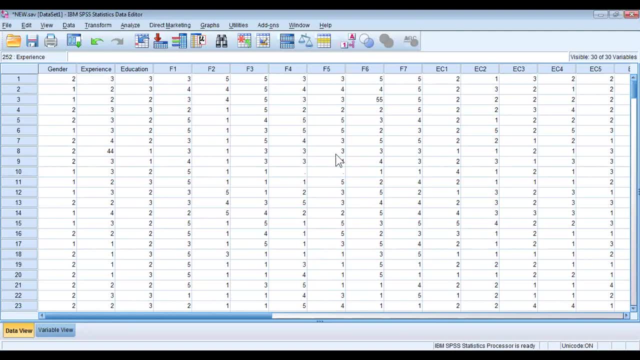 of the times, make a lot of mistakes. Sometimes, when you're writing, for example, one, sometimes you type 11,, sometimes you miss a bar, For example, if you can see here, if you've seen the last videos, it should be very clear to you that we do not have any option, which. 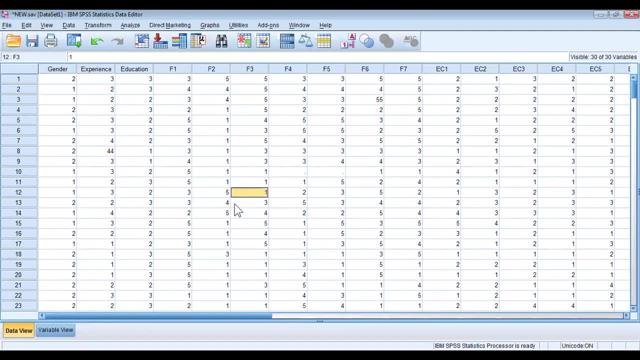 is exceeding five, that we have not coded any item, uh with a number more than five. But as you can see here that there is a 44 number, there is a 55, and there might be a few more numbers. but by visually looking at the sheet it is kind of impossible, or? 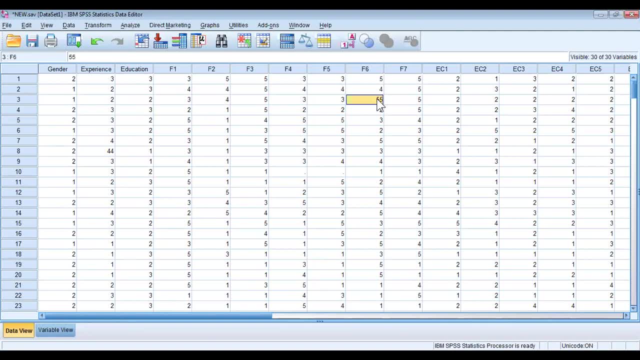 it's very difficult to uh find out all the typos. Then you can also see there are some missing values. but you, you won't be able to find all the missing values in a data. This is a data of 250 respondents. There might be a research in which, uh, you have a data. 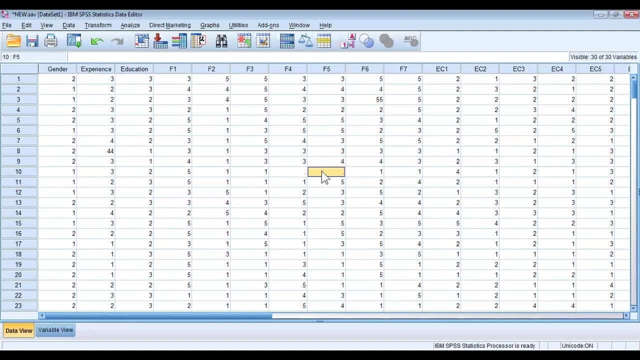 of thousands of people, So we cannot do it visually. Therefore, in this video, we'll be talking about first how to sift our data, how to clean our data, that it is a typo free. It is the error-free data. 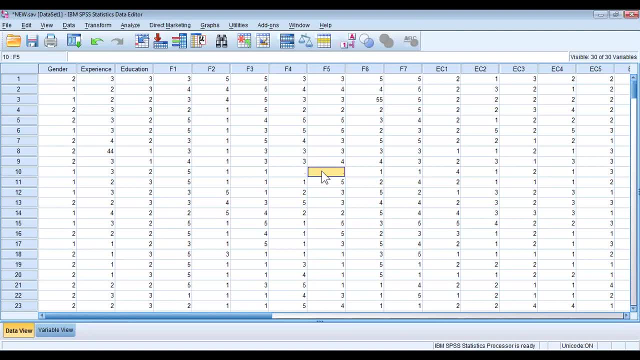 It is not going to be In part of your analysis. it will not be used in any of your analysis. You won't be putting, uh, the sifting part in any of your tables, for example, but it is a very, very useful. 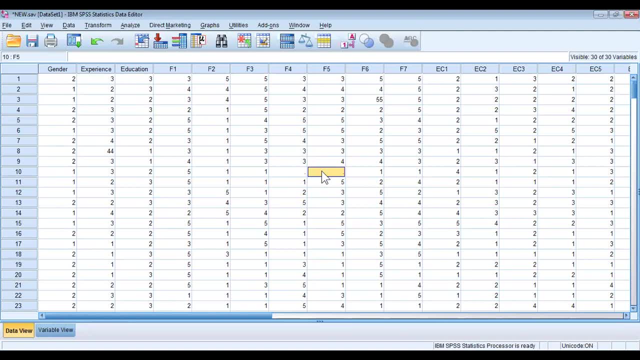 thing to do it before you move on to some important data analysis steps, because otherwise the data will be saying something else which the actual data or the respondents did not mean to say it. Therefore, let's start And, as we talked about in our presentation, we're going to talk about how to clean our 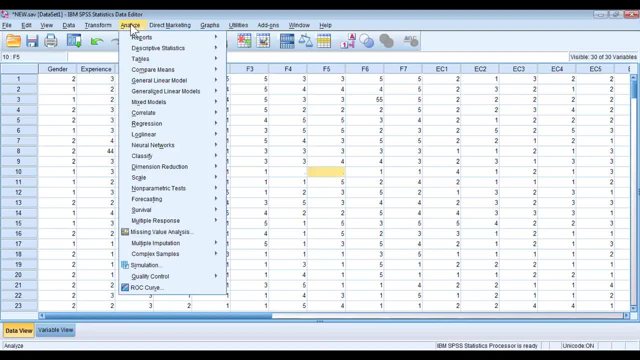 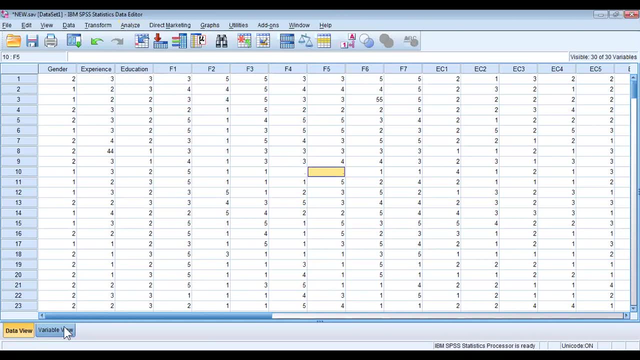 data. So in our first video that the analyze tab is going to be the most useful tab for most of the analysis. So first of all, make sure that you are in the right window. although you can do the analysis from both the windows, from both the windows you will be getting the same. 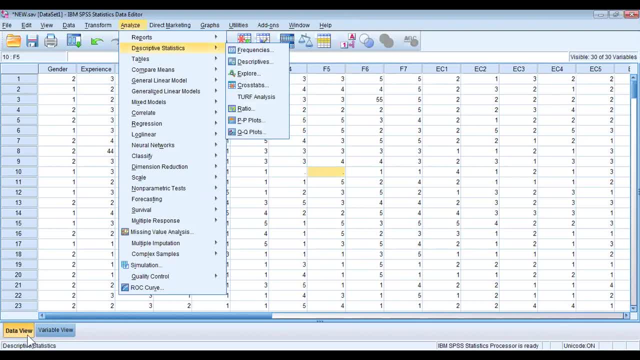 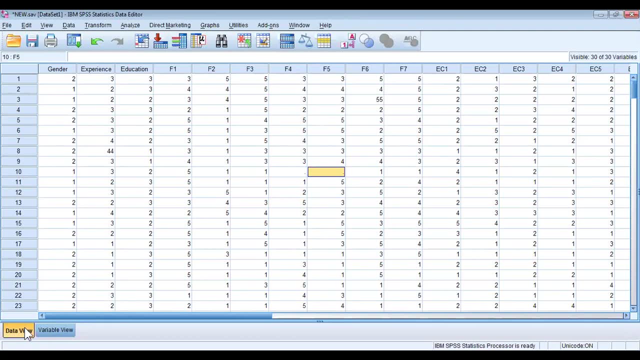 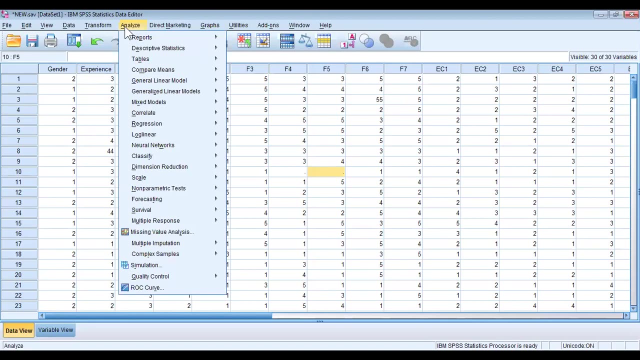 dropdown menu, but you need to be sure that in which window you are operating So you'll be performing a proper function. So let's go to our analyze window and see that there are so many options there. We'll be talking about many of these options, but for now we'll be going to this descriptive. 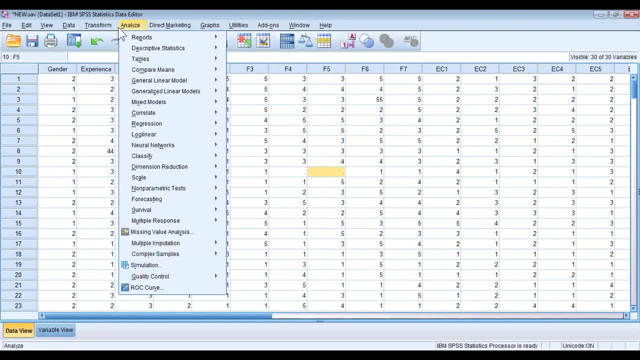 statistics tab. What we've done. we went to this analyze type drop down menu: descriptive statistics. uh, this video will contain things from the description. So the very first thing that we need to do is we need to go for frequencies. Now remember what we are trying to do. 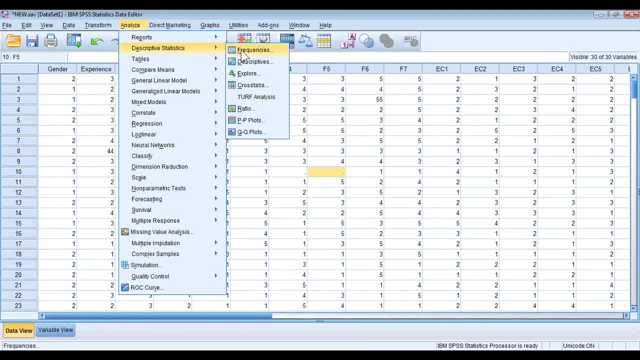 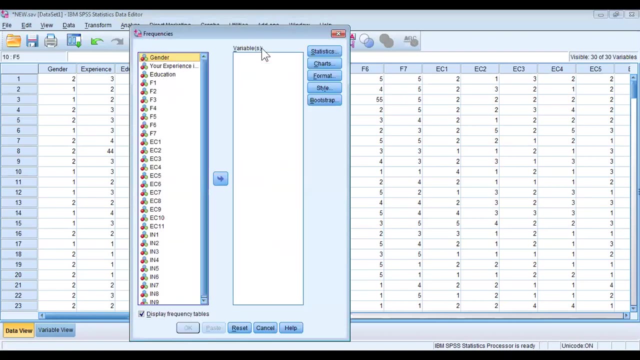 We are trying to sift our data, We are trying to clean our data, We are trying to see if there are any typos in our data or any missing values in our data. So if you just go to this frequency tab and just click it, there's going to be a new window. 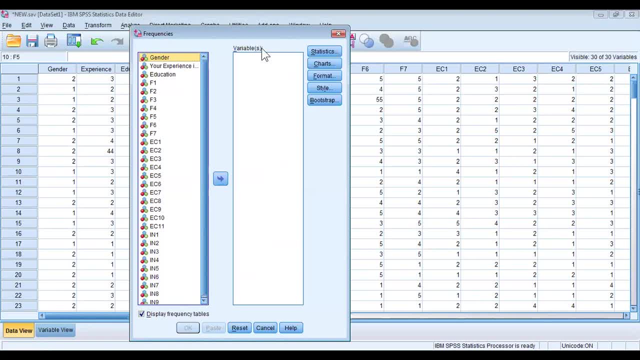 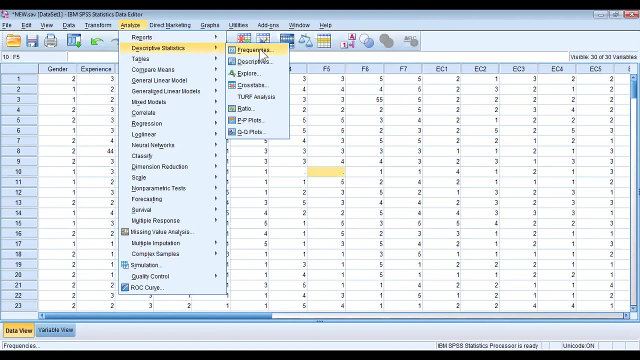 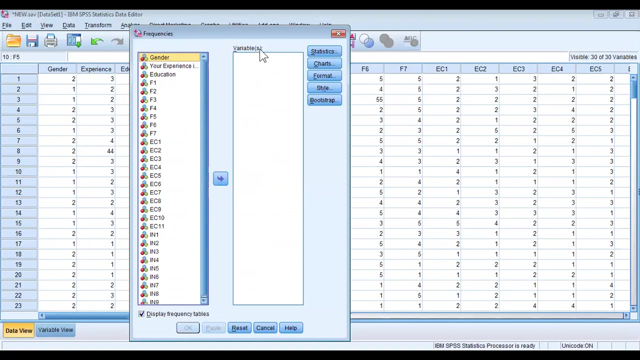 appearing in front of you. Now, this is something that you'll be seeing whenever you'll be clicking anywhere to analyze your data. What did we do? We went to this analyze tab- descriptive statistics- frequencies. So frequencies are used for many things, but for now, we'll be using it to see if our data 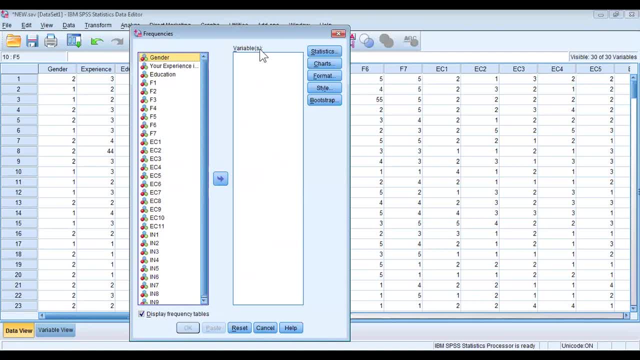 has any uh typos, any missing values? Okay, Okay, Okay, Okay. So, for the cleaning purposes, what you can do is: first you need to understand that there is this tab and there is this tab. The top of the tab is going to show you what exactly you are going to do. 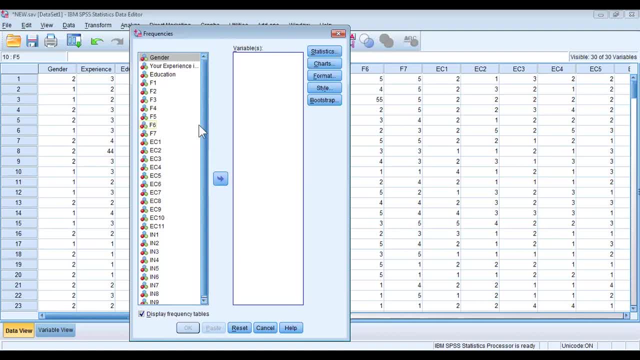 So this is a tab of frequencies. Now, these are all the questions, or this is- Oh, I have one- all the data that is available to us in our SPSS sheet, in our current sheet. So what we can do is: you can go for, for example, 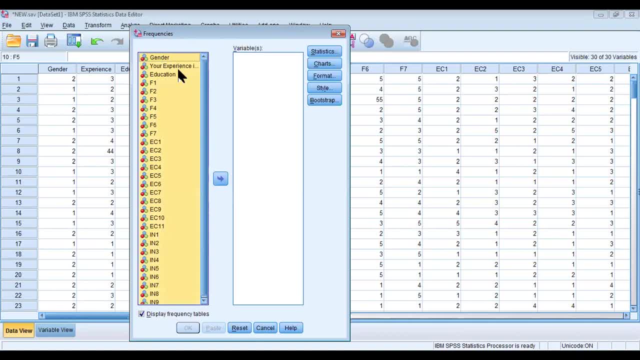 if you just click Control A, it will select all the data in our sheet, or all the questions that are there in this sheet. Now please be sure that, whichever variable you will be moving to this window, the right side window- the SPSS is going to help you analyze only these questions. 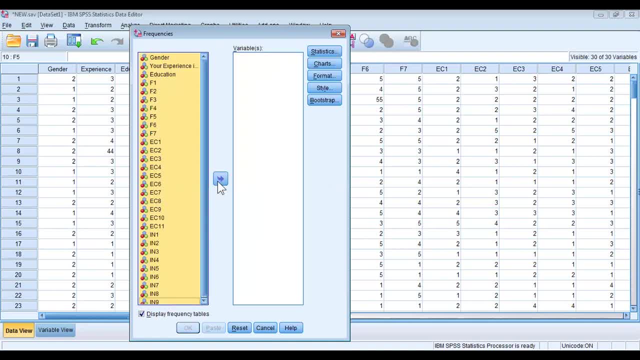 For example, you have the option to move them back, then move them here. For example, if you just want to take first three questions and you just want to sift these three, then you can move them here. So you can move them here. 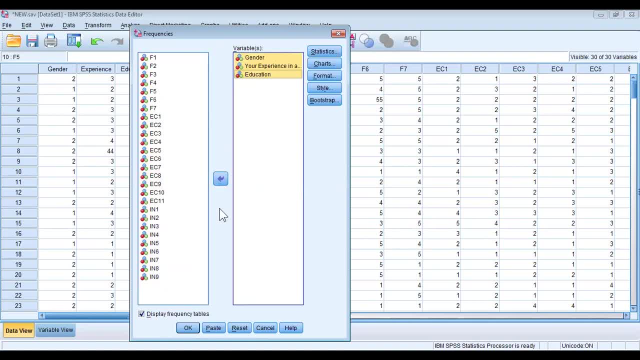 And then these three can be sifted or can be analyzed, But for now we'll go for all the variables, because what we are trying to do, we are trying to sift the data. So if you simply put all of your data into this window, 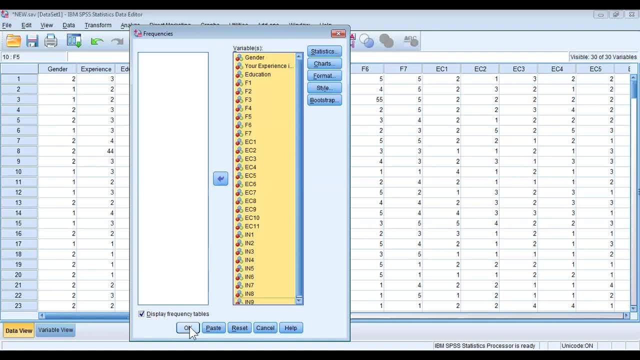 and just click OK for now. Now this is another window which is known as the output window. This is not the window which we were just talking about. So, for example, if I cross this window, it will tell me save content or output viewer to output file. 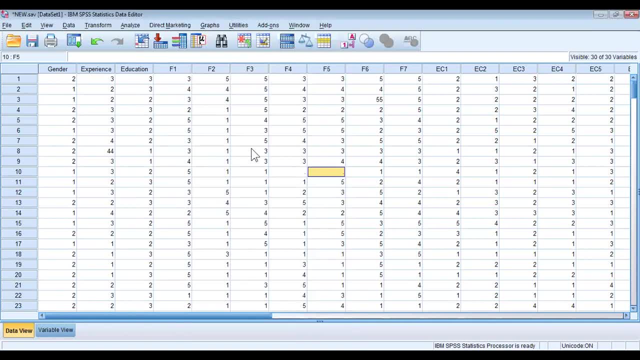 I say no, I don't want to save it. This window is still there, So make sure whatever you're doing, it'll be analyzed in a separate window. In this window we have variable view and the data view, but the variable view is not there. 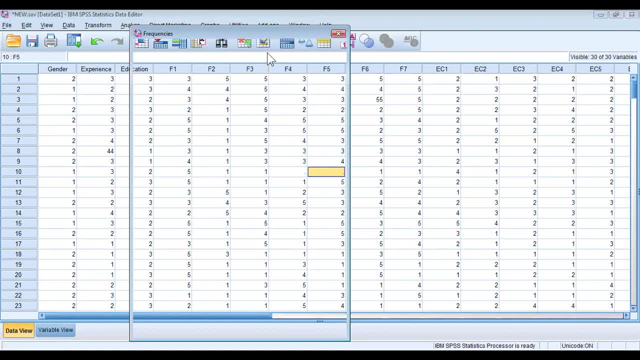 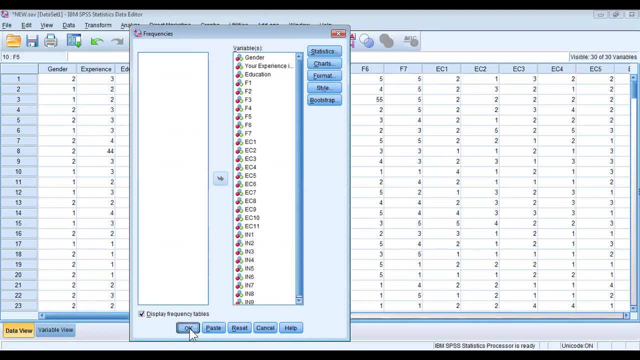 So the moment we will go for this descriptive statistics, frequencies or any other analysis, and we try to analyze, it'll give us a new window in which it is going to show us number of tables. Why? Because now, here, we can see this window now. 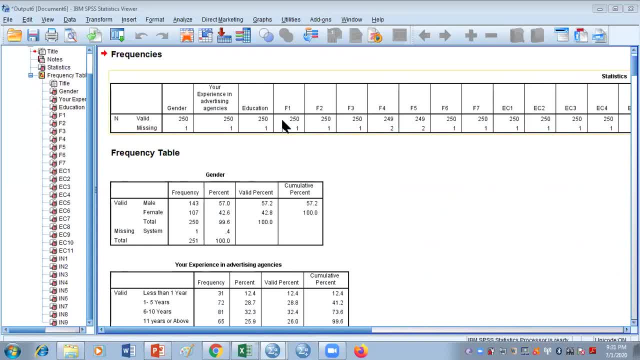 Now this window is showing us a lot many tables. Why? Because we have given it a lot many questions for which the data is to be analyzed. So if you just look at the first table, it is showing that in the gender part. 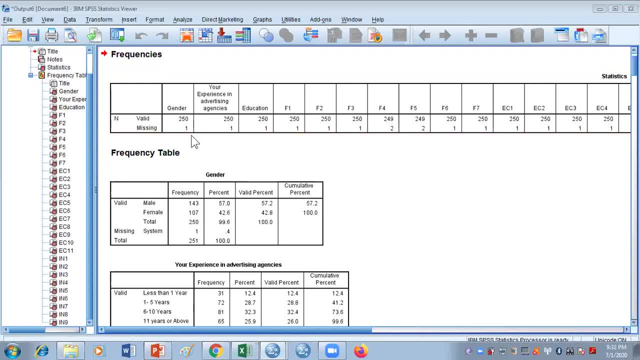 250 values are valid, which means 250 boxes are filled, but one is also missing. The same way, if we just go on 250, 250, 250, 249,, that means there are two missing values: 249, two missing values. 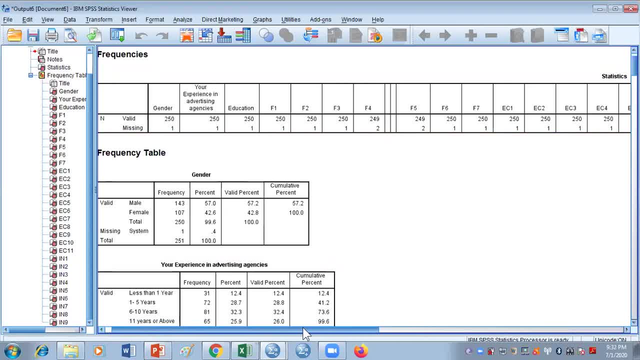 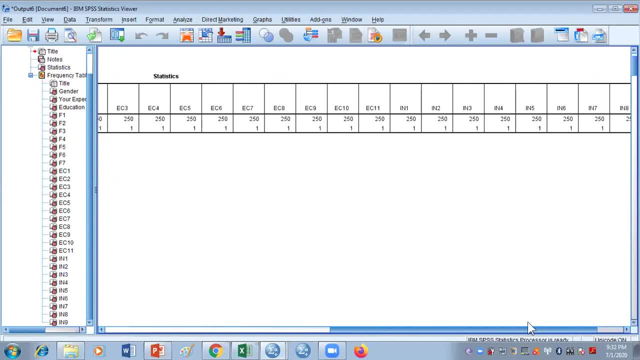 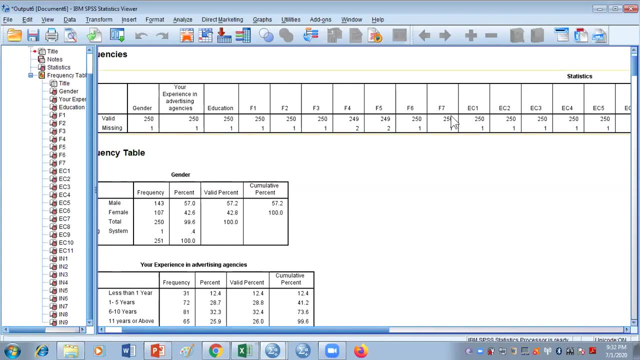 So, first of all, we will be seeing the whole data, and the whole of the data is showing at least one or two missing values. So it is showing one value missing for almost all the variables and two value missing for F4 and F5.. 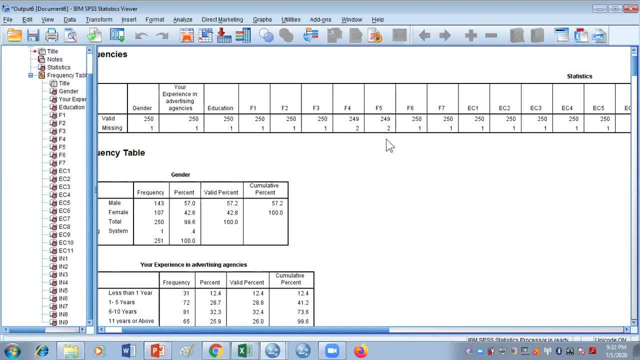 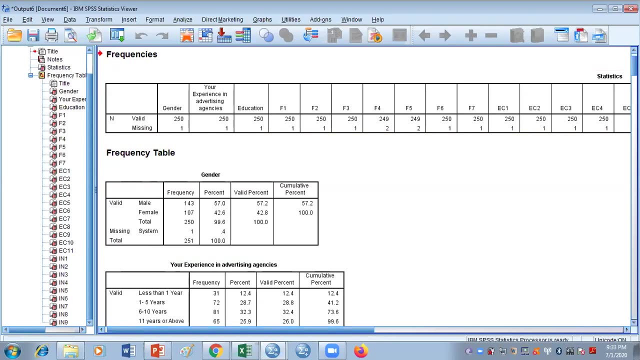 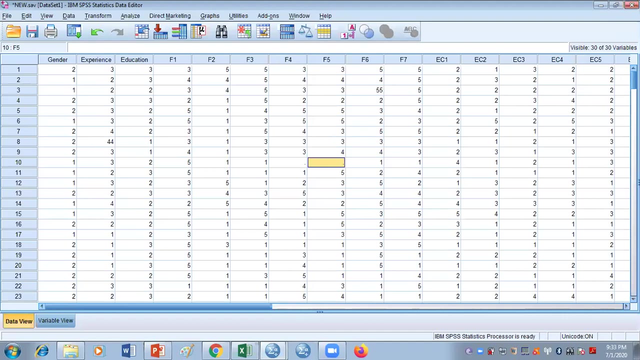 That means either respondents did not respond to this question, but the particular respondent, or we have missed the data entry. Now let's go back to our window, SPSS window, and first of all analyze that. what is that one question number? 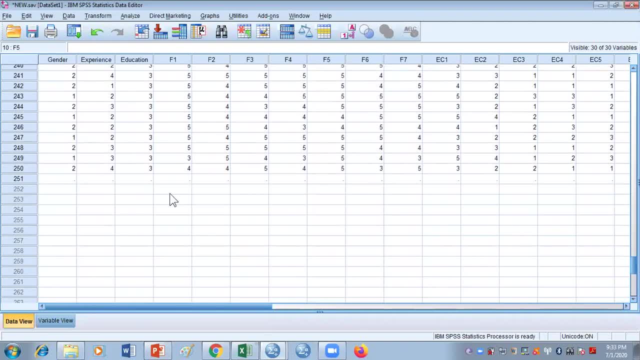 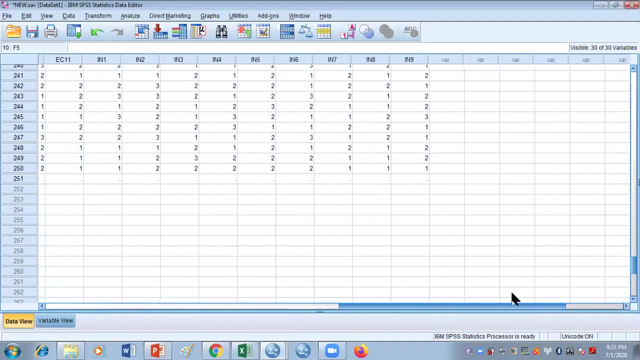 in which all the values are missing And, as we talked about in the beginning, that it is considering this 250 first line as the data and it is saying that there's no data. That is why it is showing one missing value throughout our sheet. 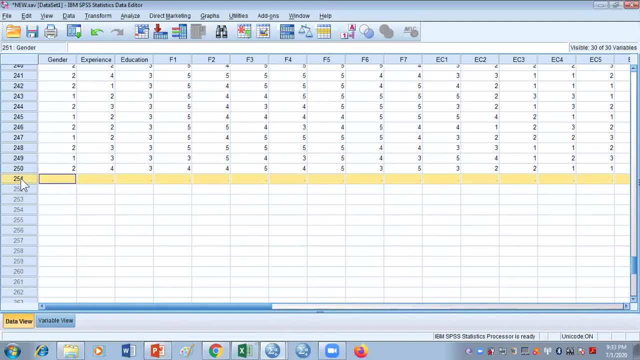 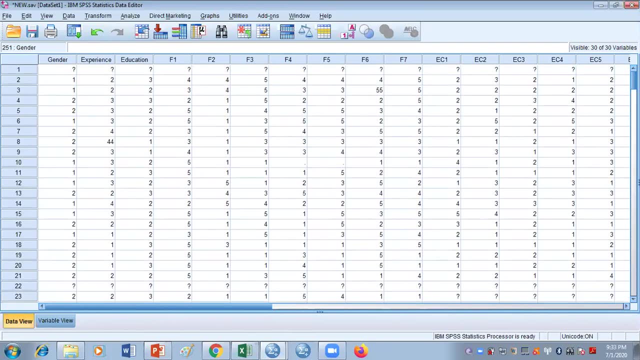 So what we can do is we can go to this 251 number right click clear. The second thing we noted in that analysis is that there are F4 and F5 missing values. So if we just scroll down to F4, and here is the missing value. 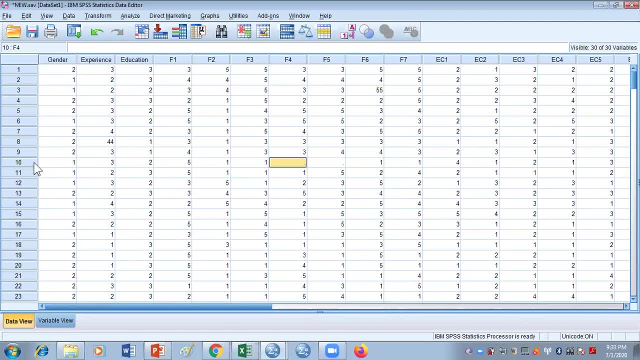 Now what you can do is you can go back to your questionnaire number one and see what the respondent has ticked in, that, For example, let's say, the respondent gave us two here and three here. You cannot just put this data like this. 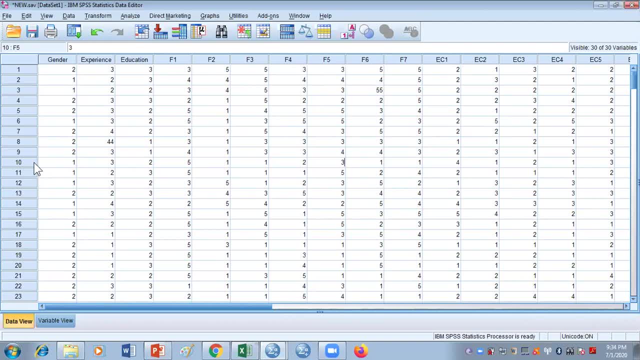 There are methods. even if there are missing values, you can use those two or three methods which we'll talk about in some other video to fill this data. But even if you leave it missing, most of the analysis will be done. 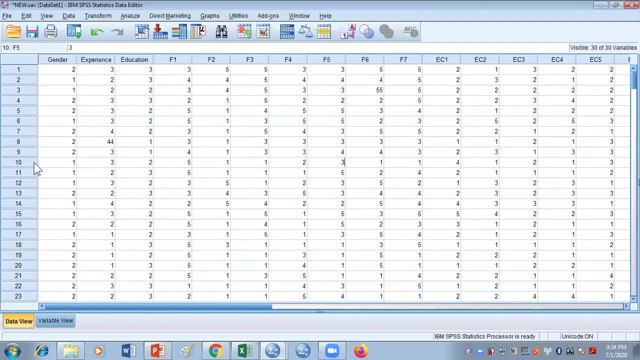 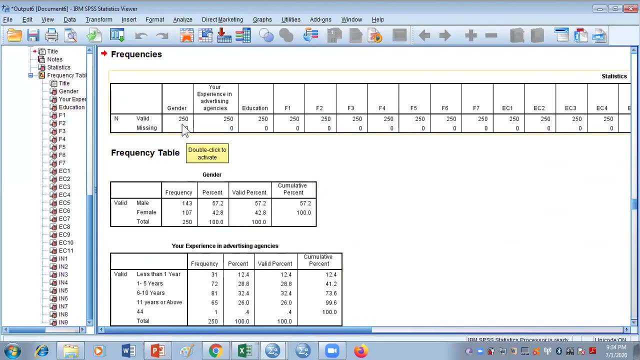 and it will not give you any problem. So this is the first thing that we did. Now let's go back to our analyze descriptive statistics frequencies and let's run the whole thing again Now. this time, what we can see is that there are 250 valid values. 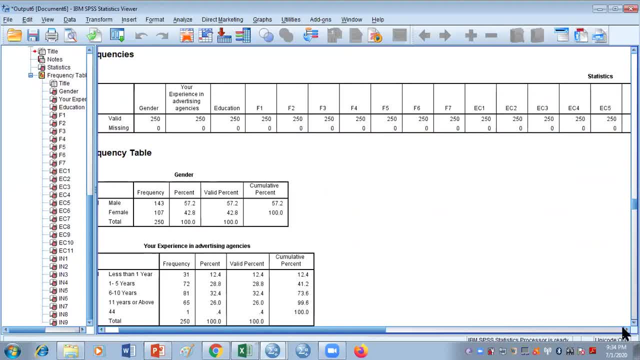 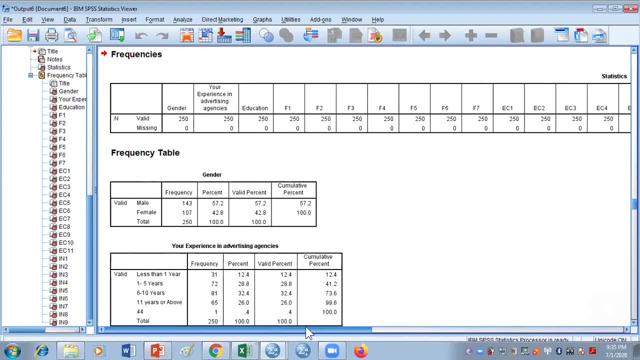 and there are no missing values. So that means with just one or two clicks we have a complete picture of our data, that there are no missing values. But this is not enough. This is not the whole sifting part. What you'll have to do is: 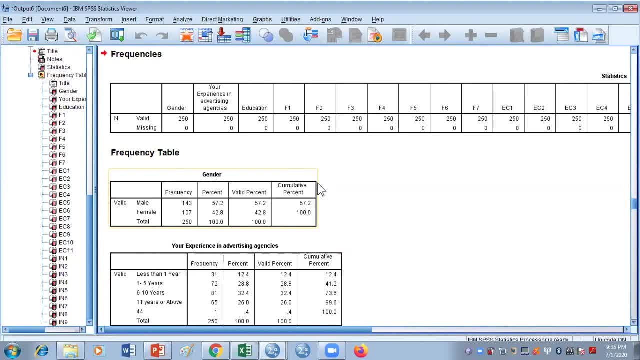 you'll have to look at the individual question. For example, here in this gender question, we only had two options, male and female, which is fine. We only have two options. In the experience part, we had these four options: one, two, three, four. 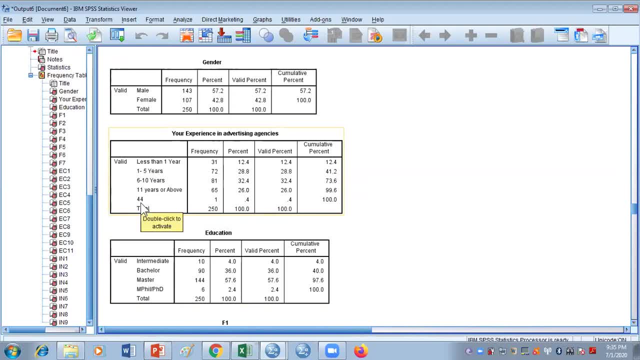 But you see there is this 44, which is mentioned, which is not part of our coding, But it had been mentioned somewhere in our sheet, in the experience row, but only there's one typo. So this is definitely a typo. 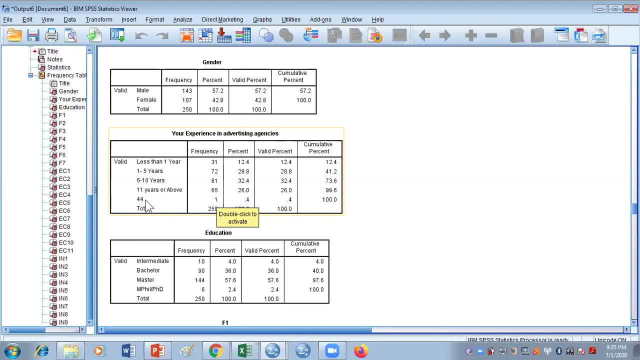 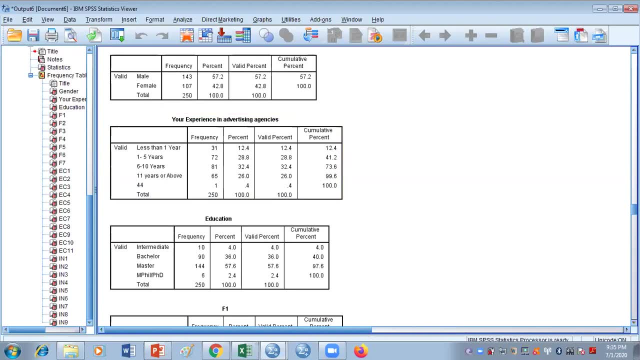 This is definitely an error, because we had nothing which is coded as 44 here. Now there's one problem with experience. Let's go to other questions. This is fine, because we had only four options, and only four options we can see. 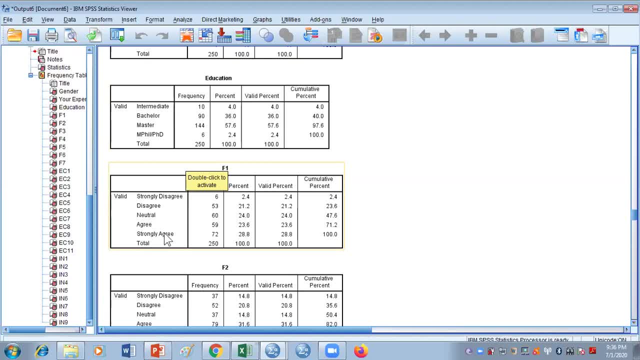 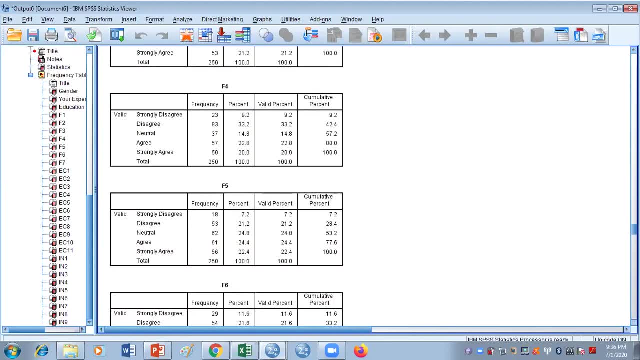 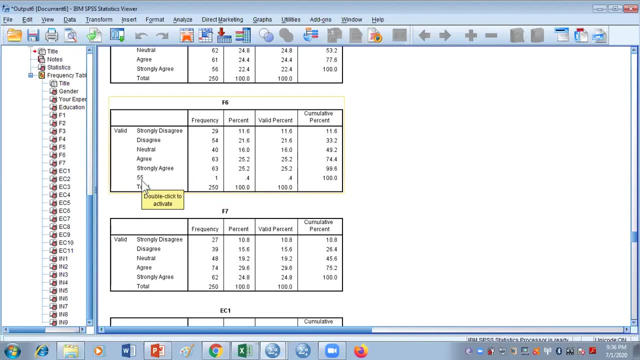 We had only five options: from strongly disagree to strongly agree, That is fine. And if we just keep on going and F4, F5, F6 here, F6 has another issue, F6 has something which is 55.. 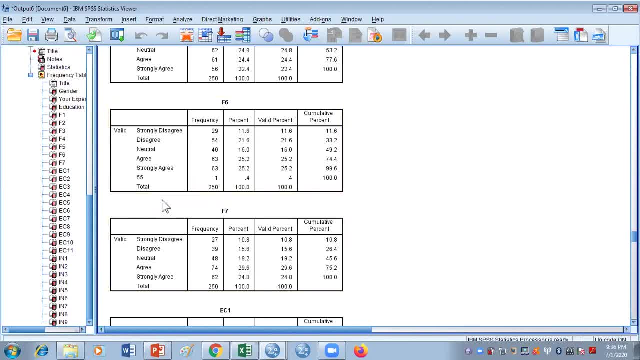 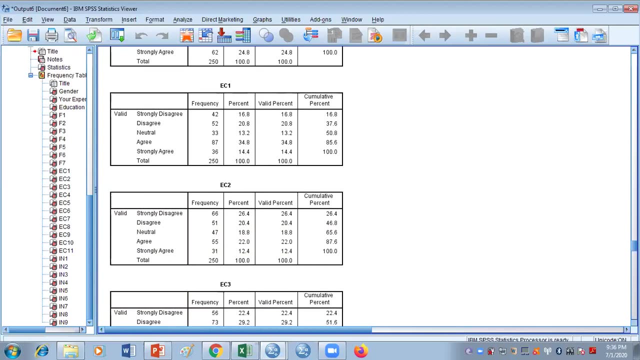 And, as we coded, the maximum number is five. Now you can easily recognize that you have mistakenly put 55 instead of five, But it's not the problem. Next, if you just look at or skim all the variables and what you can do is: 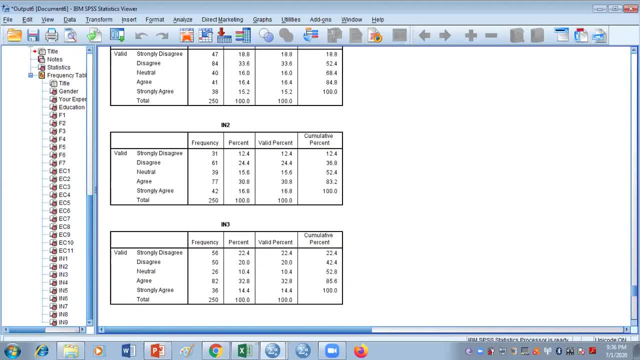 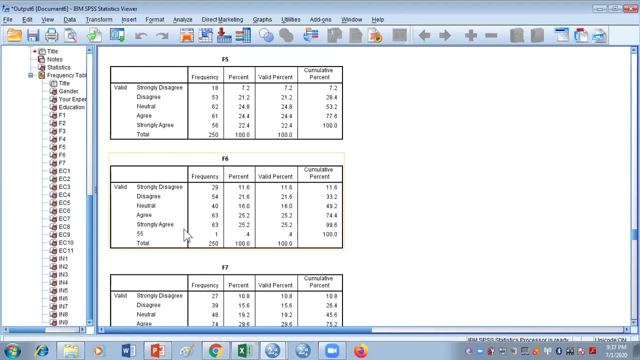 you can note down your variable number or the item number in which you have some typos. I think we are fine with the rest of them. I did this typos deliberately because I wanted to go through this step. So let's. F6 is a problematic. 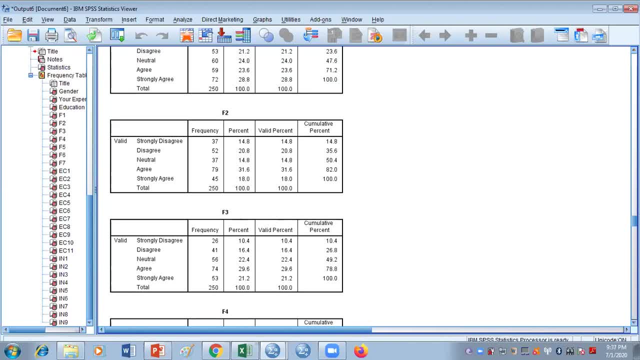 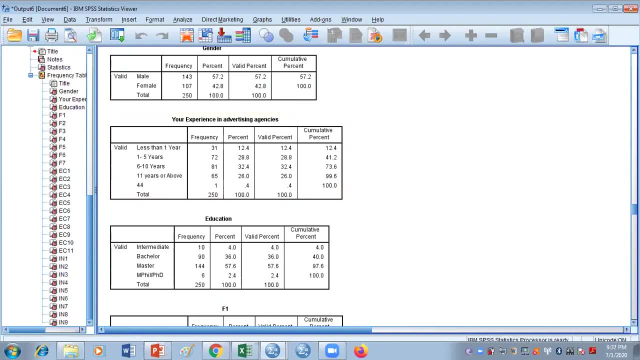 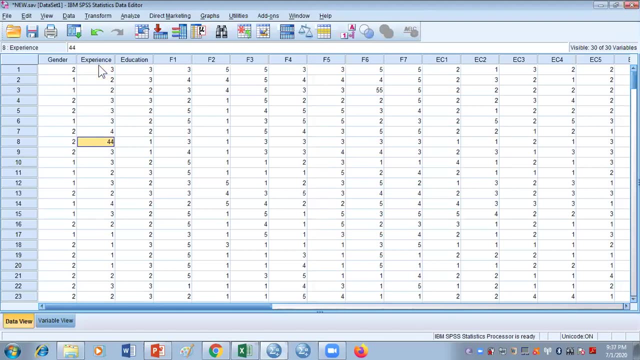 Then there is another problematic thing, which is F6, and the other one is experience. So F6 and experience. So let's go back to our window, the data view, and see experience, And here this is the typo that we made. 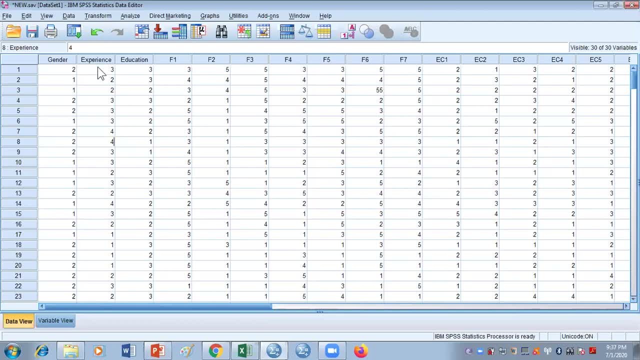 And we need to convert it to four, or we need to see what was the option ticked in. ticked in questionnaire eight. The same way, if we go to F6, and here, if you just look at this, there is a 55.. 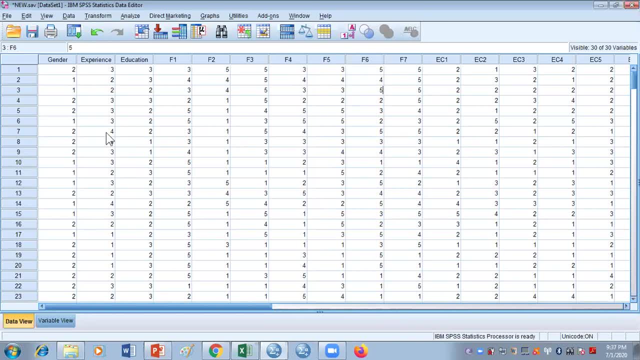 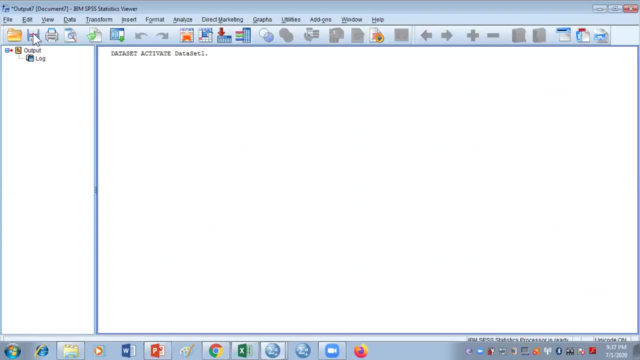 And because there is only one 55, and there was only one 44,, so there were only two mistakes in our data. So let's just save it And whenever you will be performing any function, this output window will be telling you. 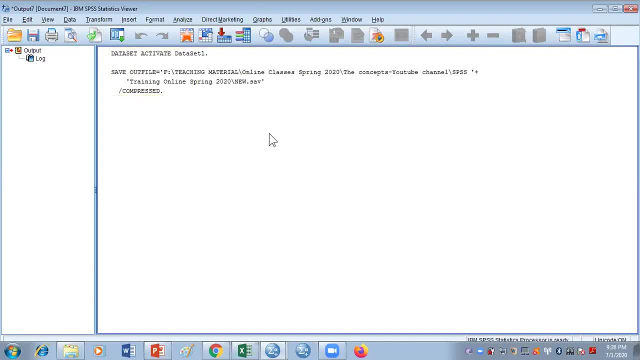 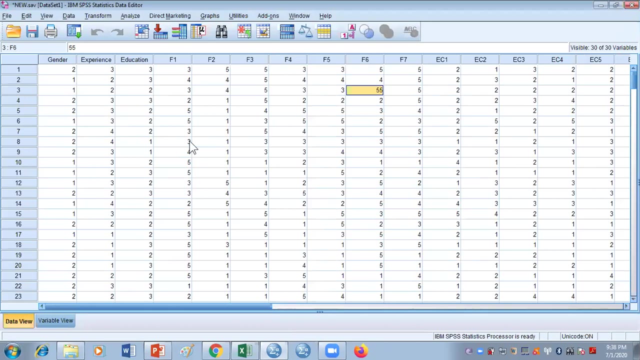 what you actually did. So if you just saved it, it's going to give you this message that it has been saved. Okay, let's close it and go back to our sheet. One other thing, for example, when I was doing this: 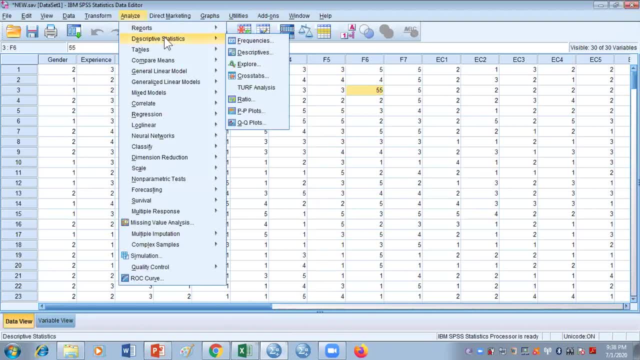 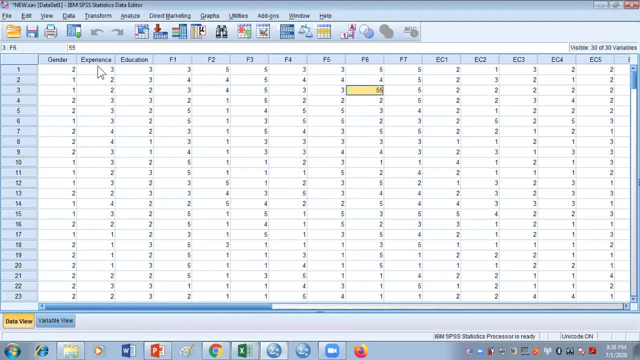 I was going again and again from analyze to descriptive statistics, to frequencies, and then I used to go to this window. There is a shortcut available in this SPSS that any recent function or analysis that you've just performed, you can just go to this shortcut. 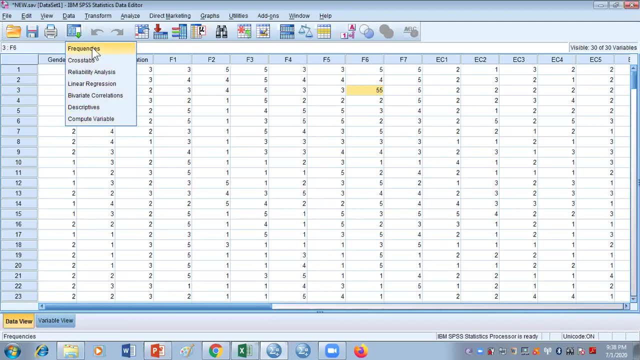 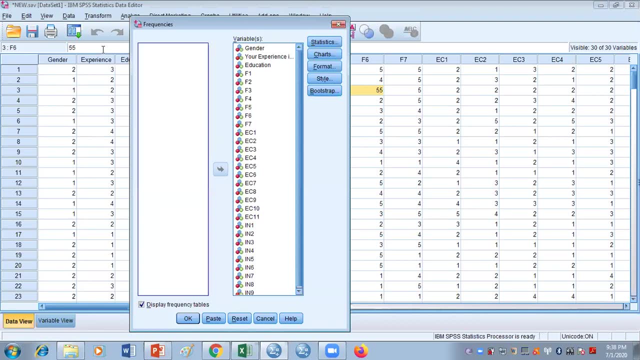 And these are all the recent analysis that I have done And, as I've recently done, the frequencies: that is why it is on the top, So just click frequencies. it's going to take you there. So, instead of going from analyze. 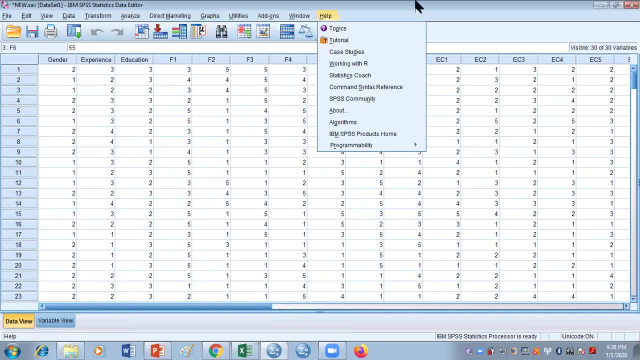 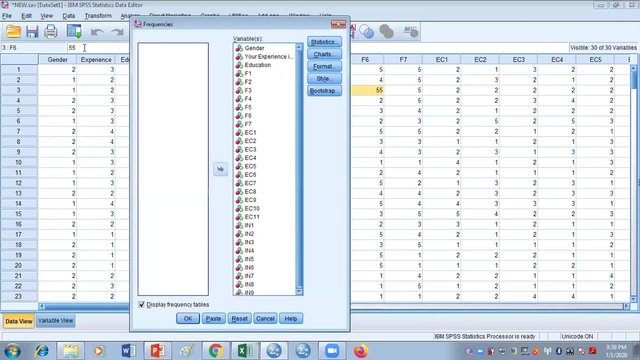 descriptive statistics and frequencies. you can just click this shortcut and it's going to take you to the frequency window directly Now, from here and from onwards, whatever analysis we'll be doing, suppose if you come here and you see that there are problems. 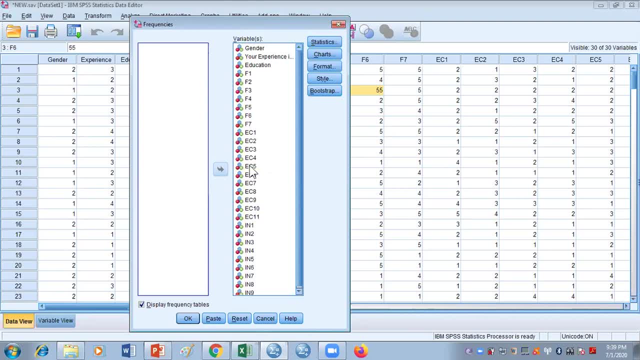 and you just want to analyze a few questions and not all the variables. So one method is that you select the variables that you don't want to be there in the span and shift them back. But sometimes, sometimes there is a chaos. There are a lot of variables. 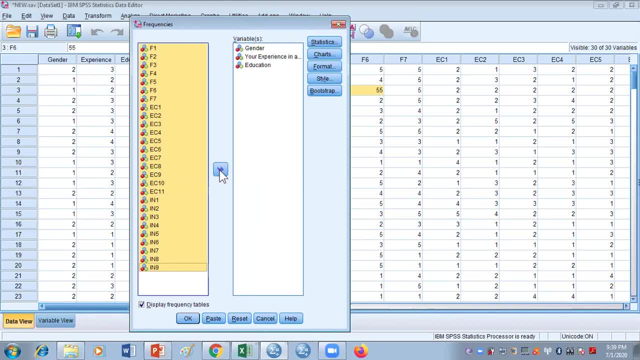 some of them you want to keep, some of them you do not want to keep. So what you can do is you can simply press the reset button and it will give you a fresh window. as a new window, Now you can shift any type of variables. 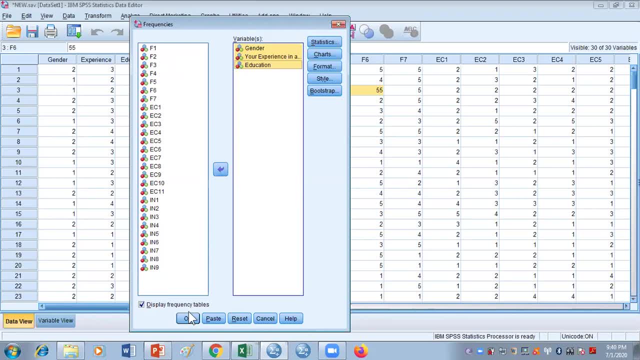 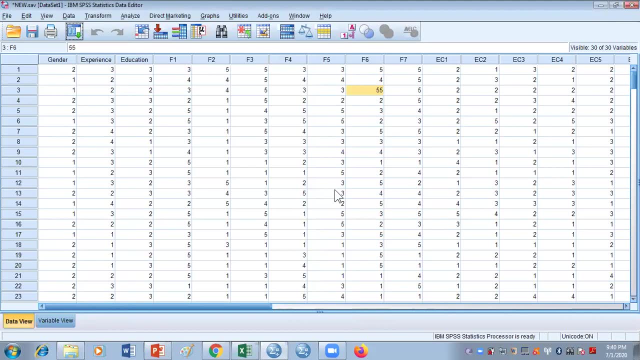 to this window and you can do the analysis Now. the frequency tab is also very useful for the demographic analysis. First we use it for the shifting part, Now we can use it for the demographic part. That how we can know that what kind of respondents. 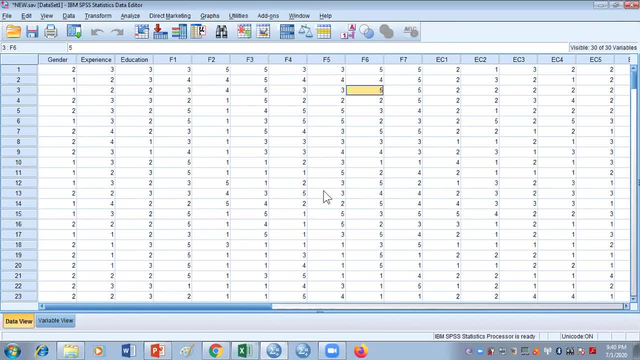 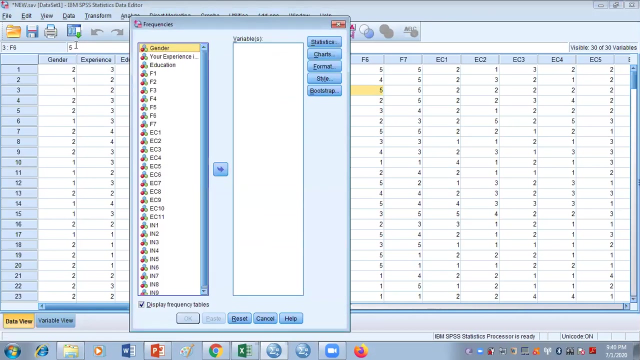 actually filled our questionnaires, And this is very important. Usually the first part of your analysis has this demographic, or you can say sample, characteristics. So for that we will again be using frequencies, But this time as we are not concerned about all the data. 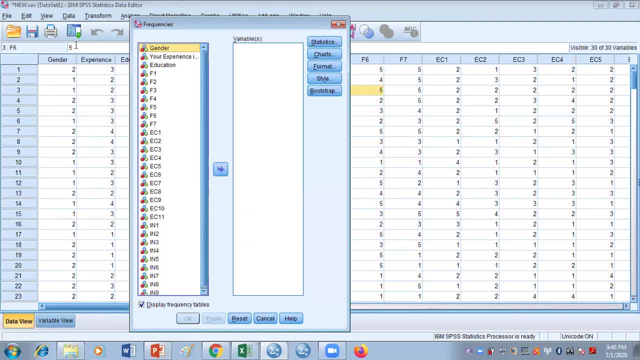 we only want to see that what was the gender, experience and education of the people who responded to our questionnaire? So we will only select these three variables And we will put them in this window Now. there are many other things that we can do here. 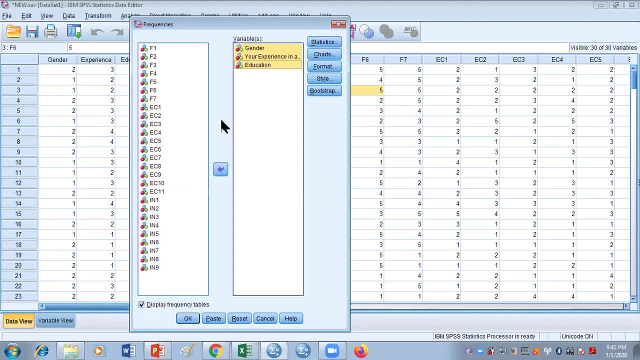 And with just one or two clicks it can give you number of different options and different analysis. For example, if you go to this chart button, it will give you option of the bar charts, the pie charts, the histograms or, if you want to see the normal curve. 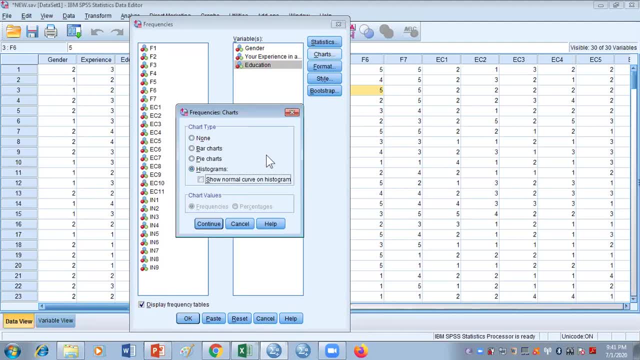 So it will give you multiple options. So for now, for example, I am interested in pie charts And I want that frequencies should be there. This should be taken as the main value, So I will just have to continue. 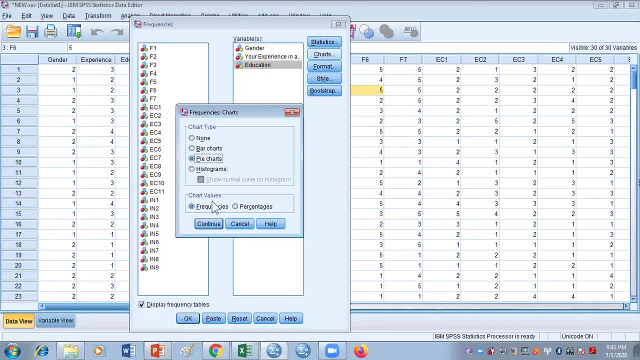 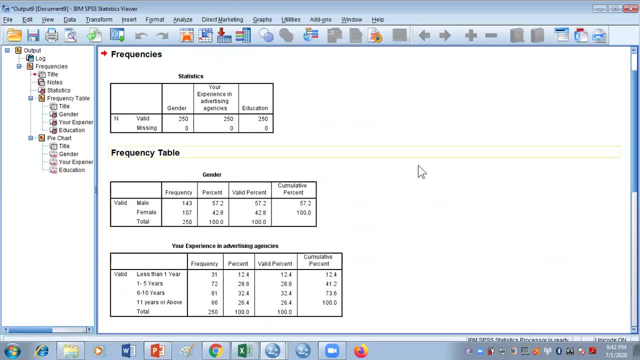 What did I just do? I went to charts- pie chart, continue- And then, if I just press OK, it is going to take me to another window, And now it is showing me. now, here we can easily do this analysis. 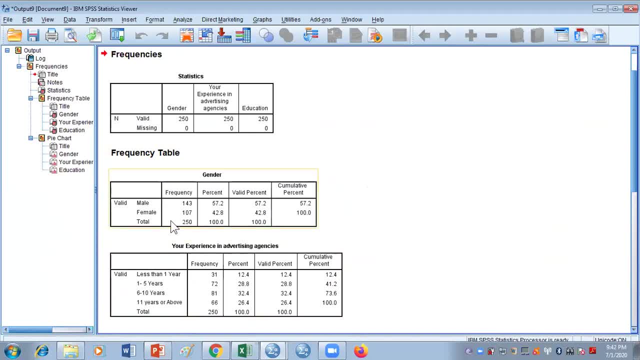 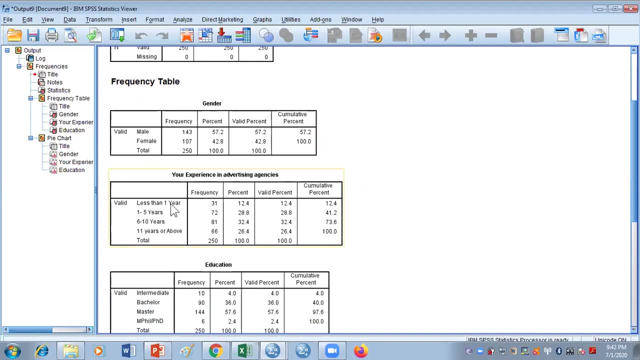 that how many males and how many females were there in our data. So 143 males and 107 females actually responded to our questionnaire. Then we are also interested in looking at their experiences. So less than one year, there were 31 people. 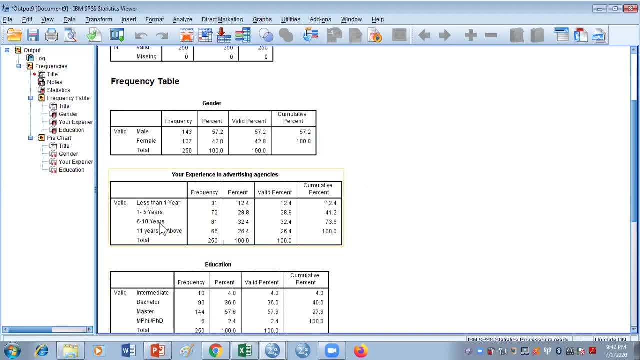 who had less than one year of experience. There were 72 people who had 1 to 5 years of experience. There were 6 to 10 years experience, which is 81 people, And there are 66 people who had 11 years or above experience. 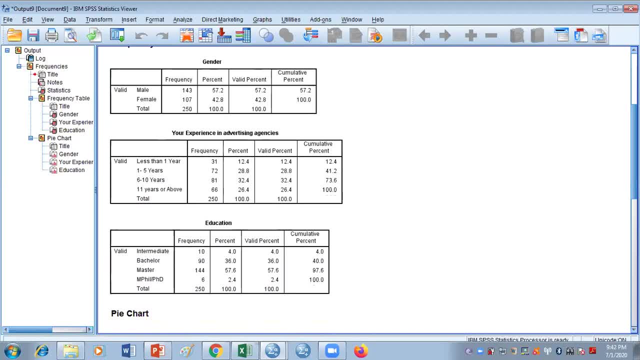 The same way, if you go to this education table, it is going to give you that 10 people had the education level up to intermediate level, 90 people had the bachelor's degree, 144 people had the master's degree and 6 had the MPhil or PhD degree. 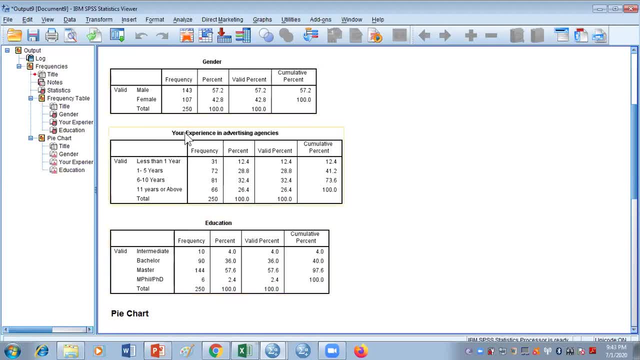 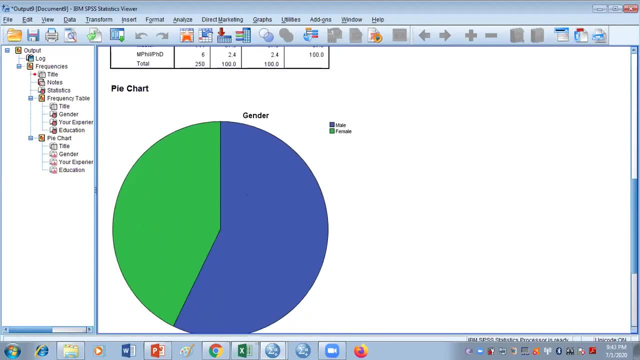 So what you can do is you can easily analyze what kind of sample was there. Now the next part is going to give you these beautiful pie charts and in which it is showing the gender, and it has divided it into two colors And the same way. 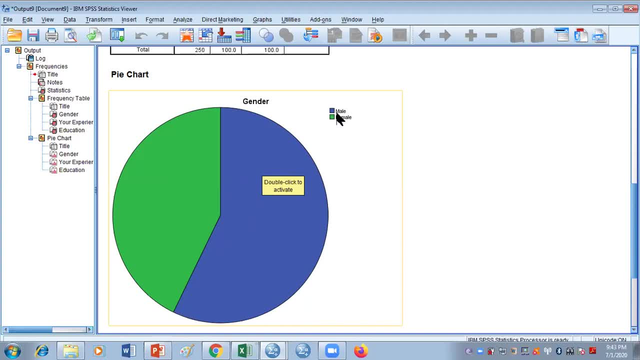 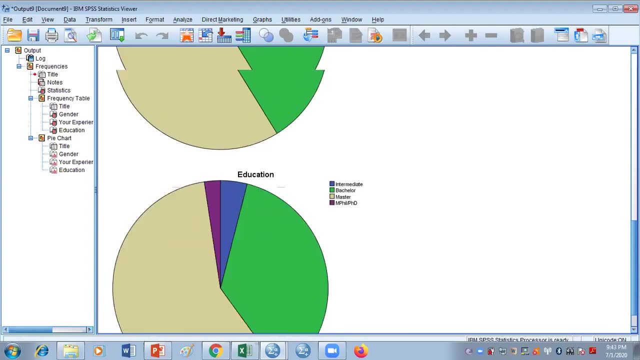 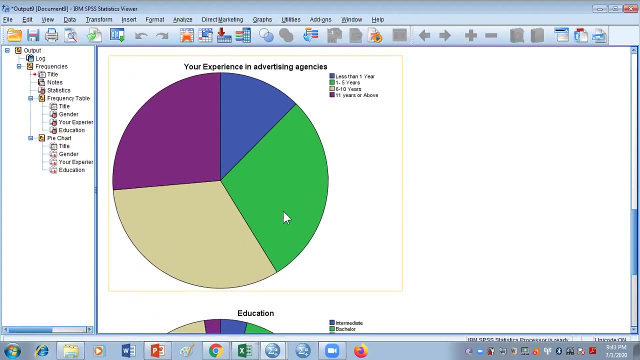 it has given you a key. For example, male for blue and female for green. Then, the same way as we had four options in experience part, less than one year, and all of them they have different colors- The same way education. 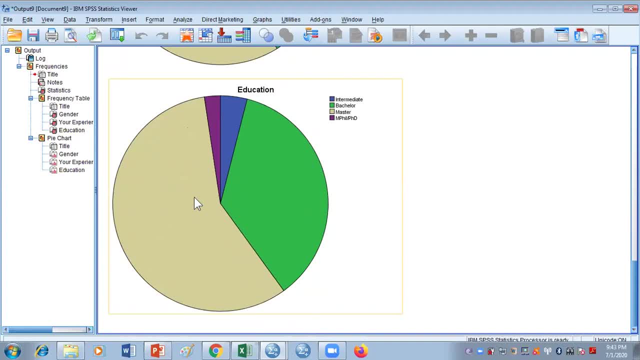 And, as you can see, that there are more people who have master's degree and there are very few people who have MPhil or PhD degree, and there are very few people who have the intermediate degree. So this way you can get very beautiful graphs. 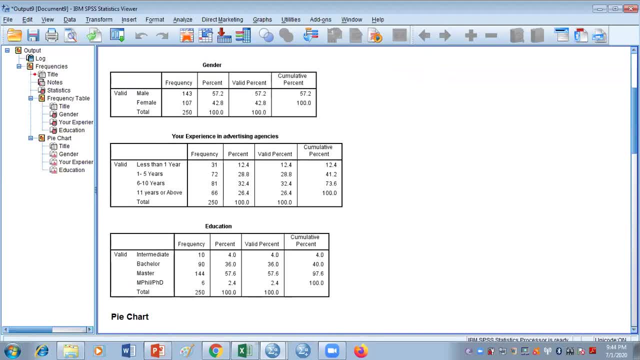 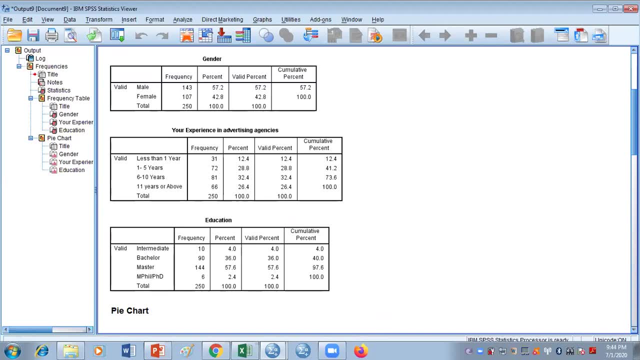 with your tables. Now I will be making other videos how to convert your tables into APA or into beautiful, presentable tables, But please never, ever, make this mistake of just copying these tables directly to your report and presenting them like this, Because 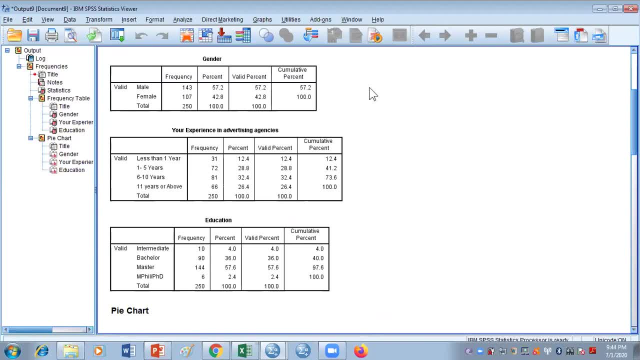 from the output window. you just have to right click, copy and you can paste it anywhere. For example, if you want to paste it in Excel, if you want to paste it in Word, you can do it. You can also. 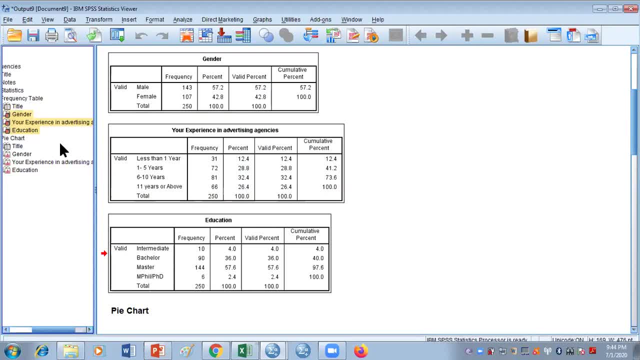 by pressing from here you can also go for multiple table selection, So you can just copy and paste it anywhere. But please don't do it. Do not just copy paste them. Make good tables, for which you will be looking at my other video. 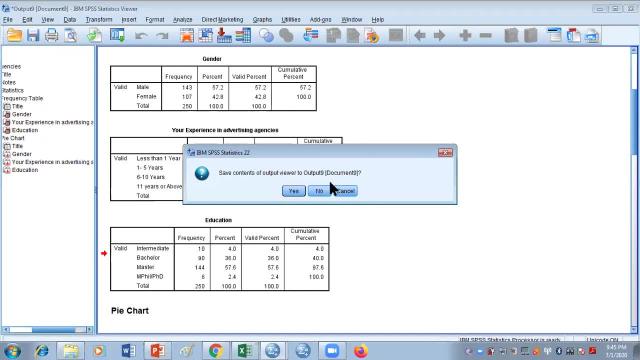 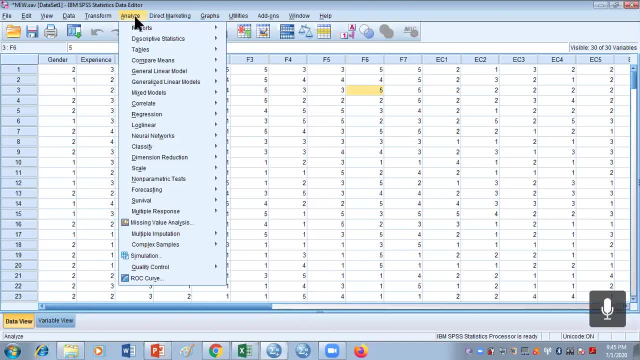 Now, the last thing of this video we want to understand is that in the analyze part, there is also one very interesting function that we can perform. Go to this descriptive statistics and go to this cross tab. We will be talking about the descriptives in our next video. 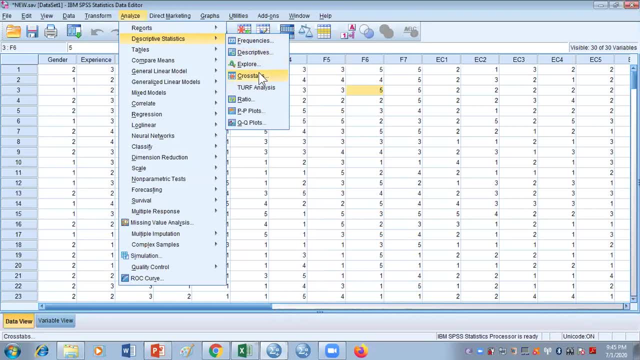 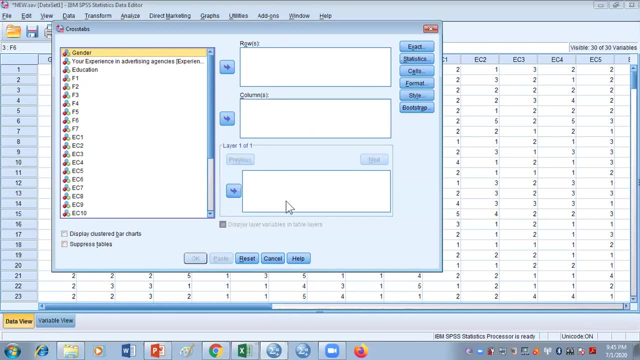 But for cross tab you need to go here, Press the cross tab. Now it will give you options of row, columns and layer. So, for example, if I am interested to know that, what, how many, for example? 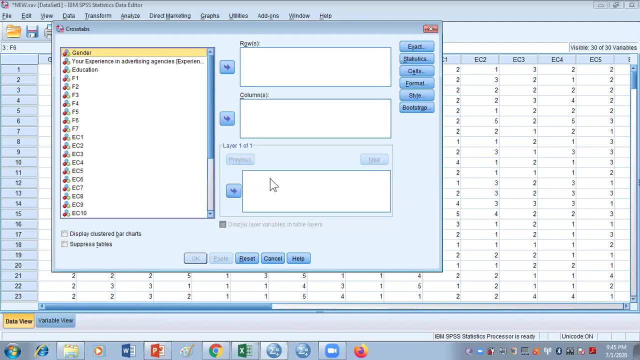 male respondents were having master's degree and how many female respondents had more than five years of experience. So the questions like that can be answered through this cross tab. So we are in the cross tab window, So what we can do is. 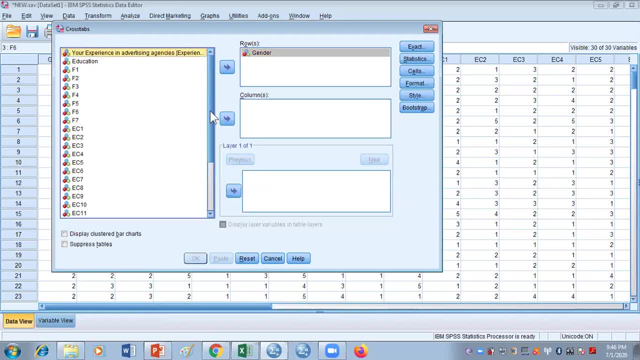 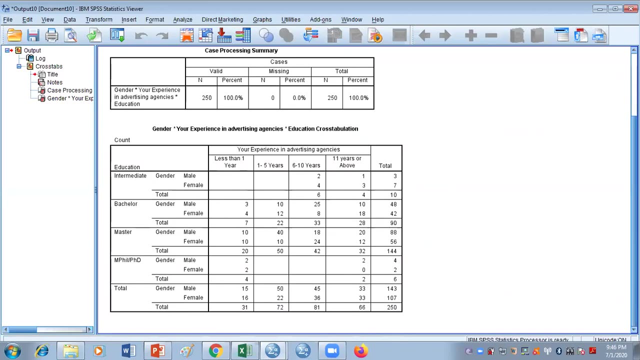 we can put gender here, experience here, and education, for example, here And for now, just click OK And what you can see is you have a very detailed table. Now, what it has done for us is that it has taken. 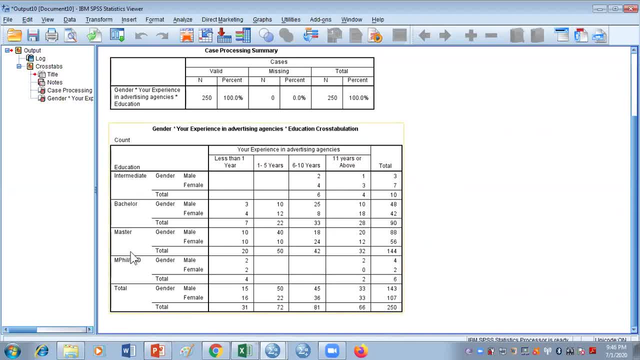 the education here, the four levels of education of our sample, the two gender types and the years of experience. So by looking at this table we can easily analyze that, for example, three male member having less than one year of experience. 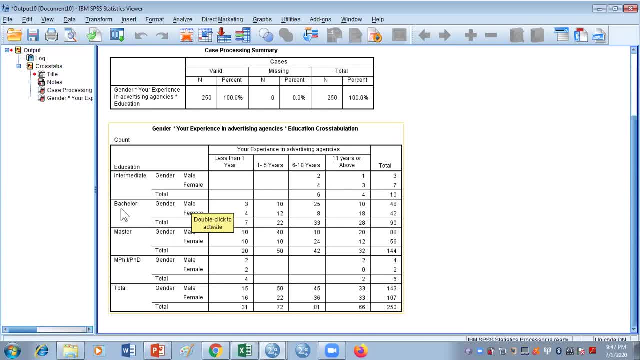 they also had bachelor's degree And, for example, how many people had, what kind of people had, intermediate degree. So there was only two people who had this intermediate degree, who were males, And there were four females who had six to ten years. 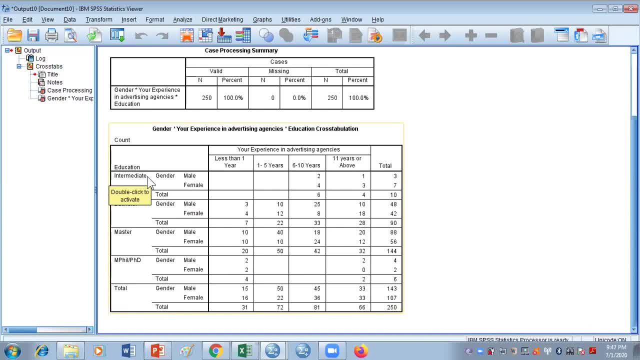 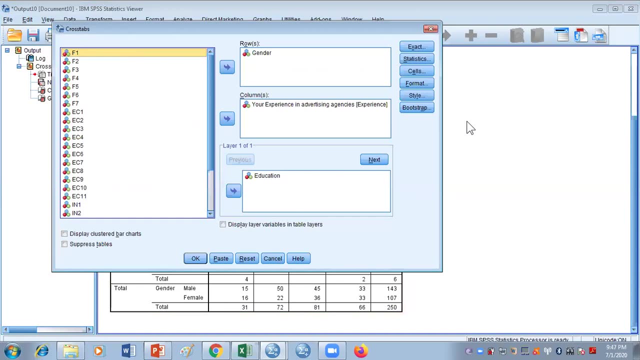 of experience, but their education level is intermediate. So this is a very, very useful tab in order to know what kind of people had what kind of other characteristics. The same way, if we go to this shortcut, again cross tab and you can also go for 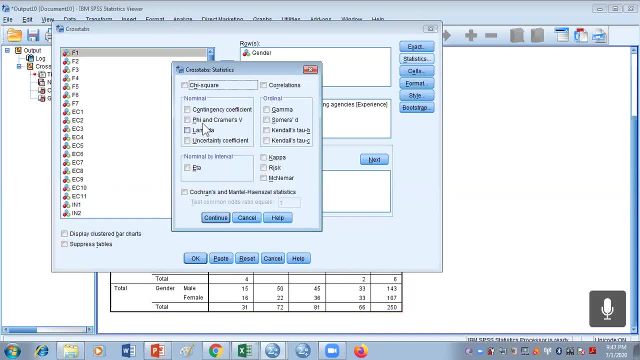 other things. for example, you can go for statistics, and in statistics you can go for many of these options which are, for now, very complicated and we won't be talking about it. You can also go for, for example, formatting of these. 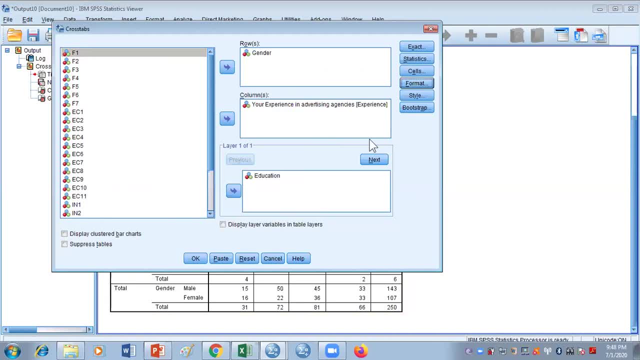 things, that if you want it in ascending order or descending order, you can also go for the style that, what kind of style you want, But all of these things are possible in this cross tab window. So this is a very 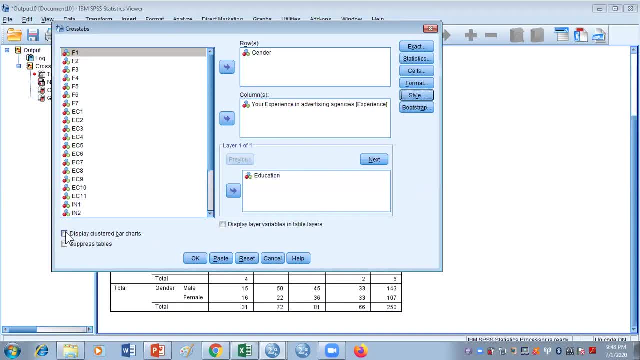 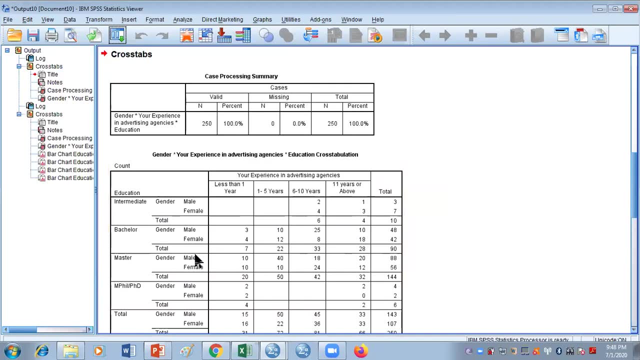 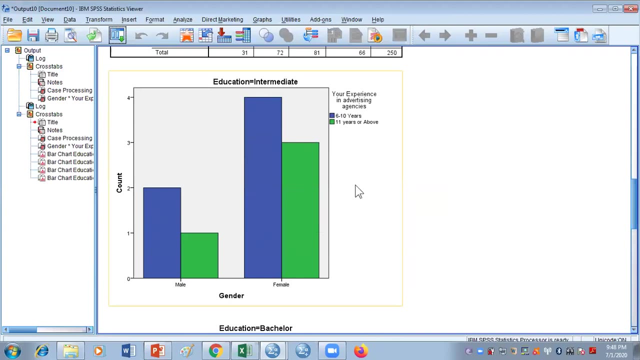 very useful window, And from here you can also go for display clustered bar charts, and let's just try this one as well. So once you do this, you will also get these very beautiful bars that are showing that female had six to. 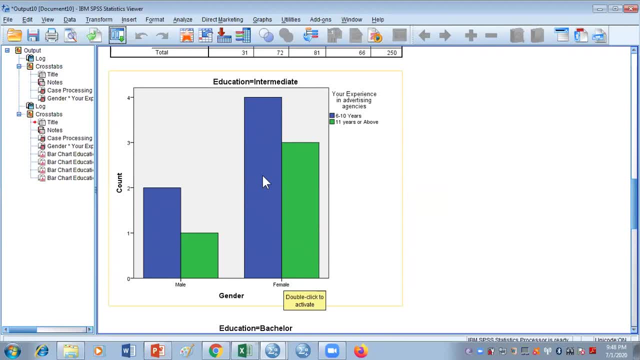 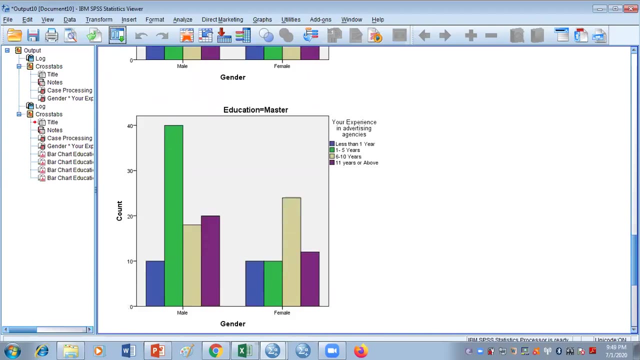 ten years experience are here, and female having eleven years or above experience are here, So you can do multiple types of analysis, and this is for gender education. this is for education and gender. this is for education and gender, So you can have multiple. 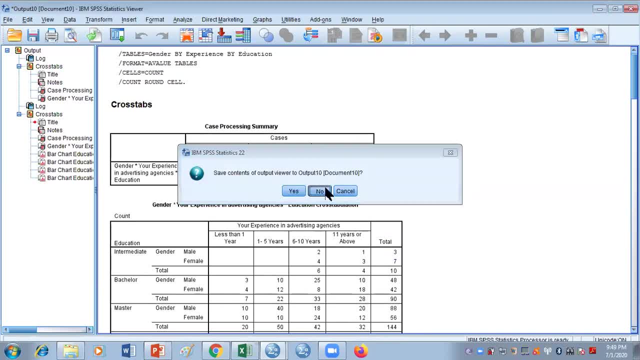 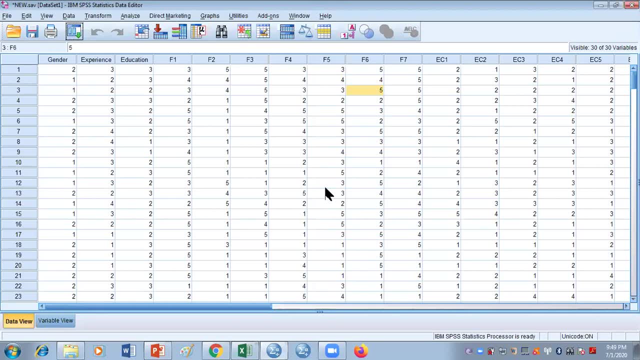 options here and through cross tabs. many of the researchers only use, sometimes, cross tabs. For social sciences researchers, the cross tabs are the only analysis that are used and the frequencies may be. So keep practicing these things and in the next video, 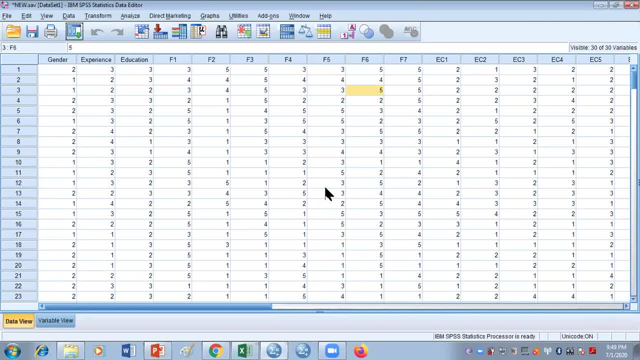 we'll be talking about some other things like descriptive statistics, and then we'll move on to our correlation, regression and further more complicated analysis. For now, thank you very much.